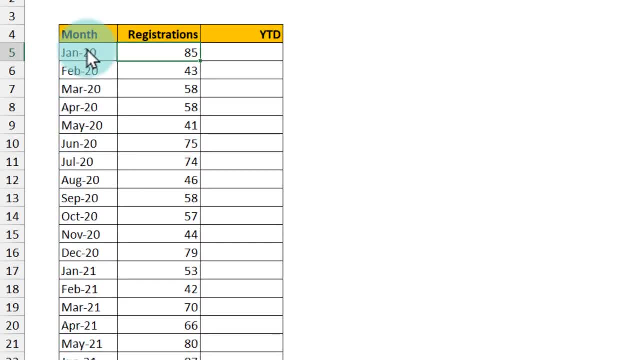 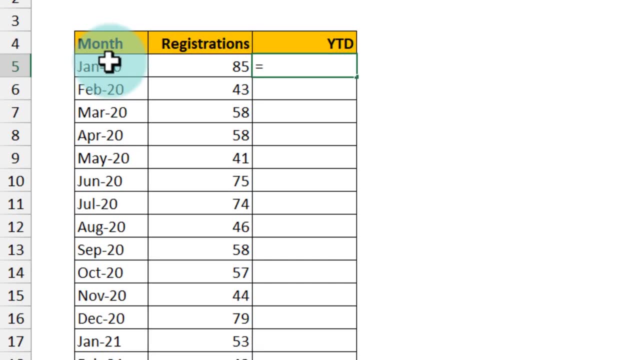 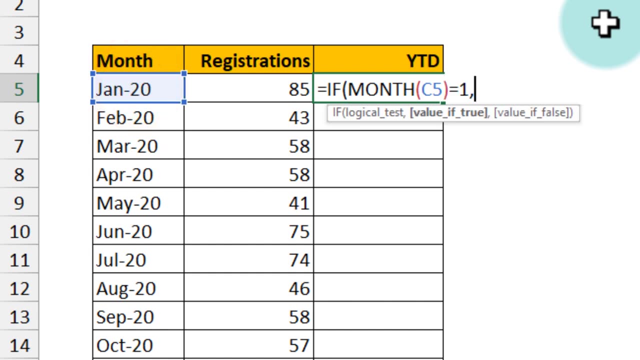 a tabular data. We're also going to look at the mythical offset formula. Watch the whole thing. We can use the if formula to set up the year to date calculations. We'll say if month of this cell is equal to one. We are assuming our year starts in January, so if it is one, then this is the value that we want. 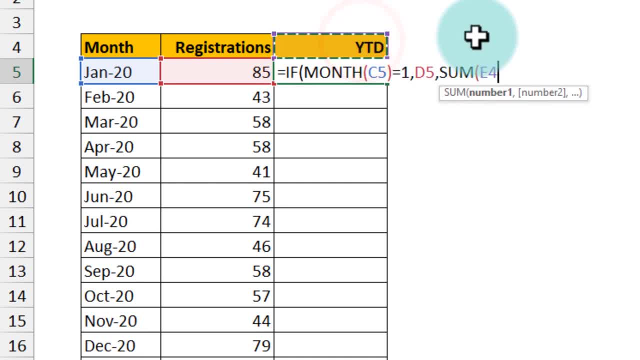 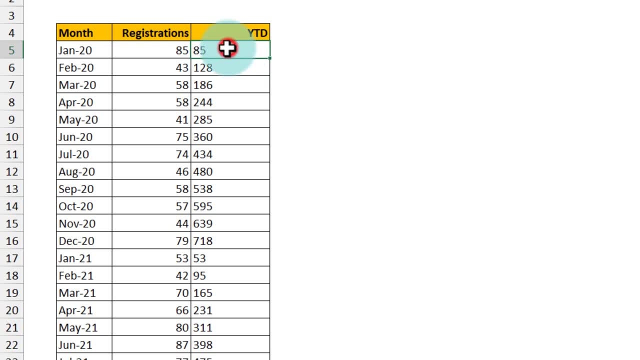 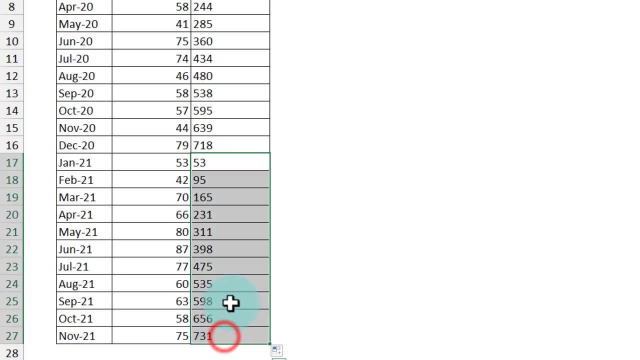 else. we want to sum up previous cell and this cell. You will understand how this works. once we drag this down You can see that it goes from 85 to 718 and once we hit January again, it resets to the value of January and then the count goes up again. How would we do that if our year starts in? 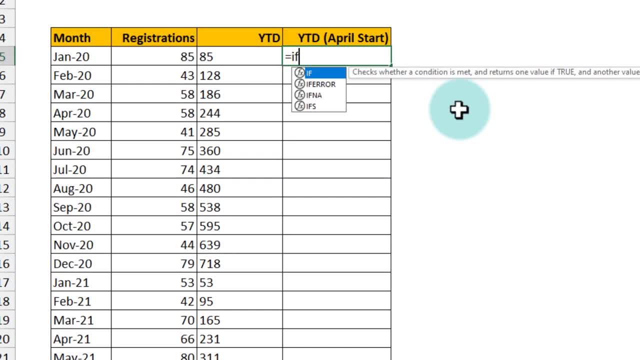 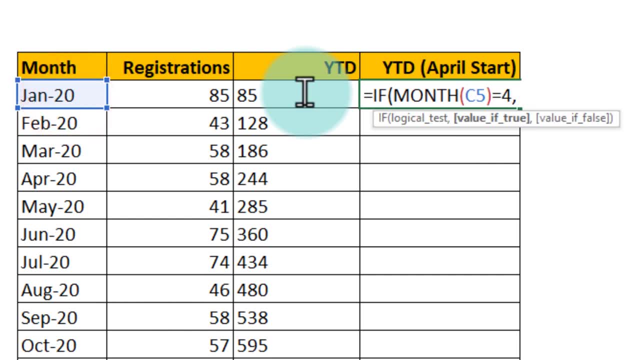 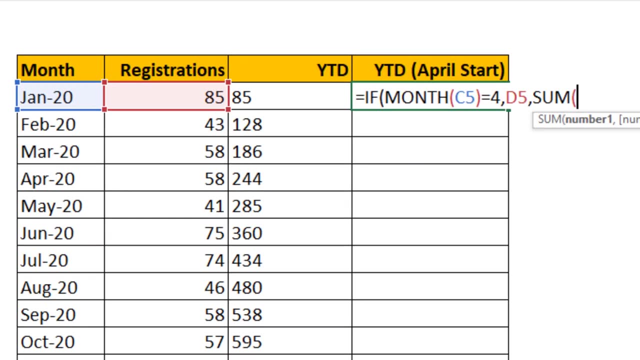 April. Let's just say April. In this case, our formula goes like this: If month of this cell is equal to four- because our year starts in April, which is the fourth month- then the value we want is in D, else sum of D5 and this value, and then we can just fill this down. 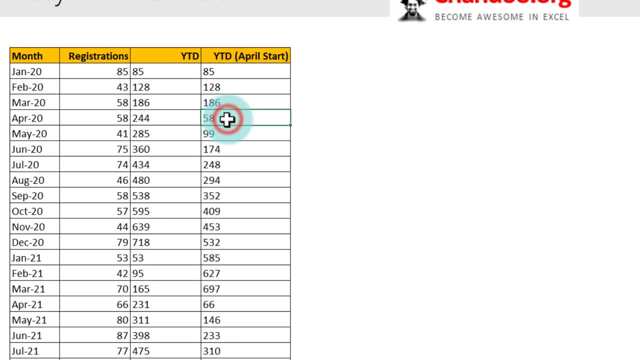 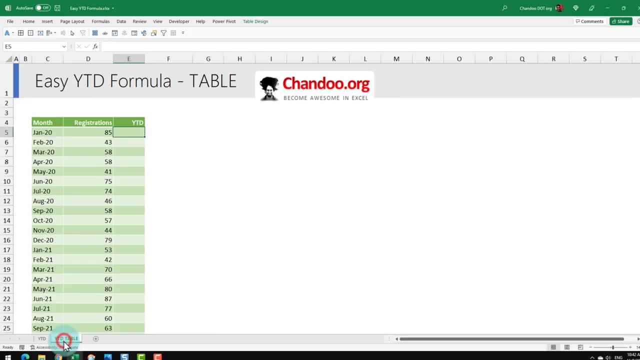 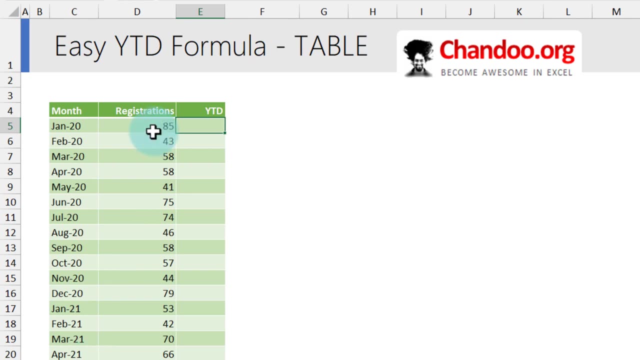 You can see that the value goes from Jan, Feb, March. In April it gets reset and then it goes again like this. Now, how would we do all of this if we have a table format of the data? The challenge with tables is because tables have the relative structural references. 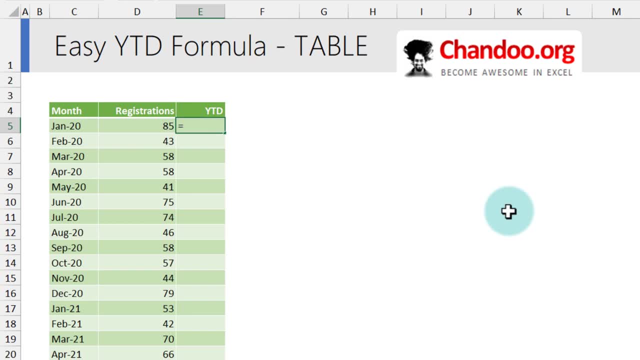 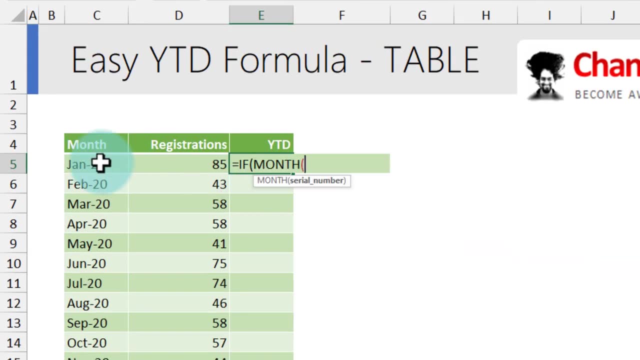 the formula becomes slightly tricky. Let's observe this. So, with year to date from Jan, the formula is: if my month of at the right month is equal to one, then I want registrations, else I want a sum of D. Now here is the problem. Our first value is registrations, but the second value needs to be: 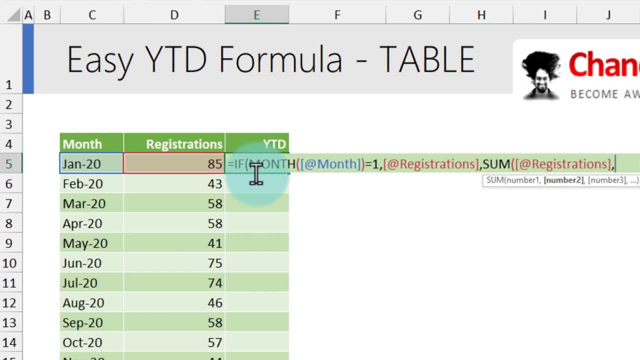 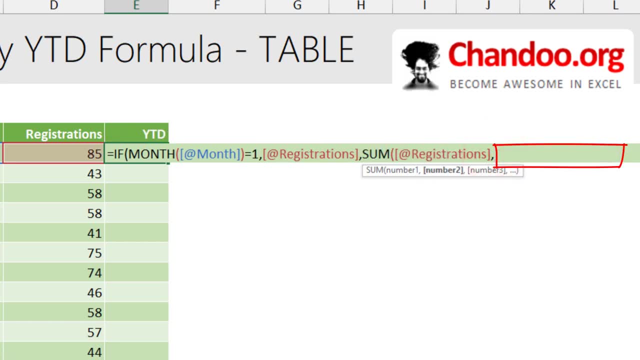 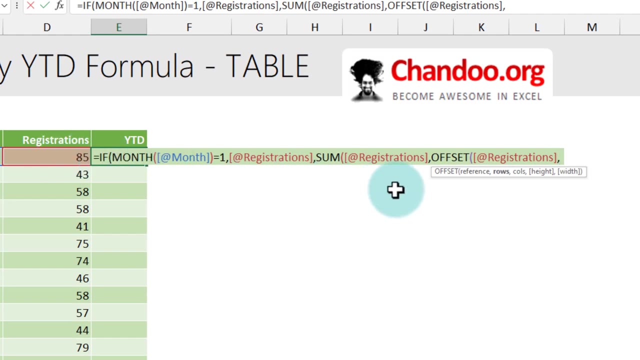 the value one month prior. You can see that the ytd column is here because we cannot really refer to this value or anything like that. This will become data headers ytd. We'll have to use a different formula. This is where offset comes in. We could say offset of registrations: go one row.